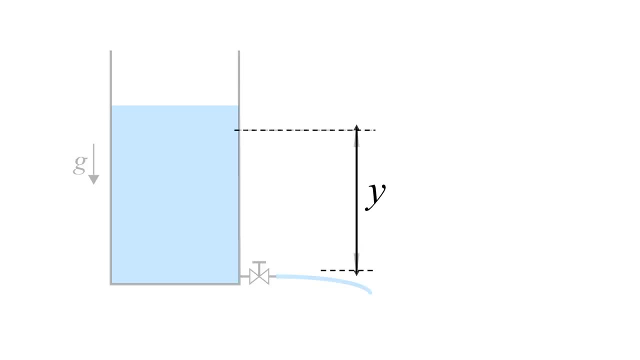 Now, when you open the valve at the bottom of the water tank, you can drain the water. One thing that I would like to highlight here is that the water draining speed is proportional to the water height. In other words, the higher water height builds the larger hydraulic pressure. 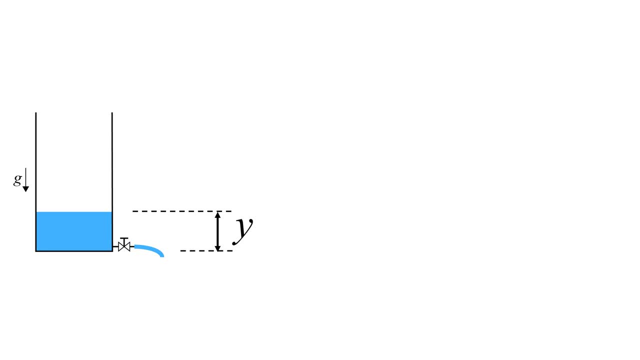 Causing the larger water drain. To mathematically describe this physical problem, you can use dy over dt for the water draining velocity. The dy over dt stands for the how fast your water height y changes with respect to time. Since the water height y decreases as the time goes by, I need to use a negative sign. 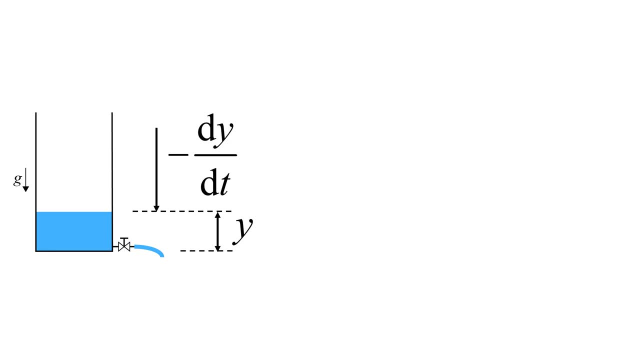 As you can imagine, the water draining velocity is the velocity of the water. Since the water drain velocity is proportional to the water height, y itself- I came up with minus dy over dt is proportional to y. To further develop the equation, we can introduce a coefficient alpha. 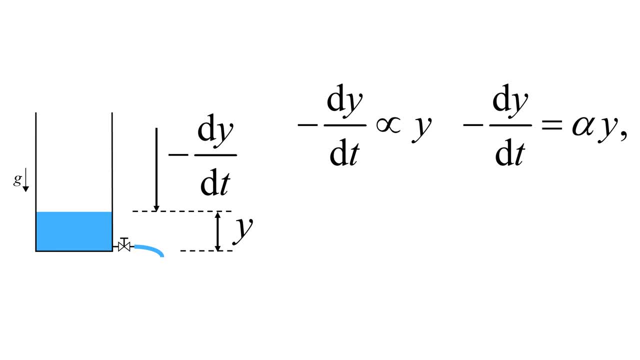 which is related to physical properties such as the water tank cross-section area, hydraulic resistance of the valve, gravitational acceleration and etc. To simplify the problem, I chose 2.. It can be changed depending on the physical system that you are working on. 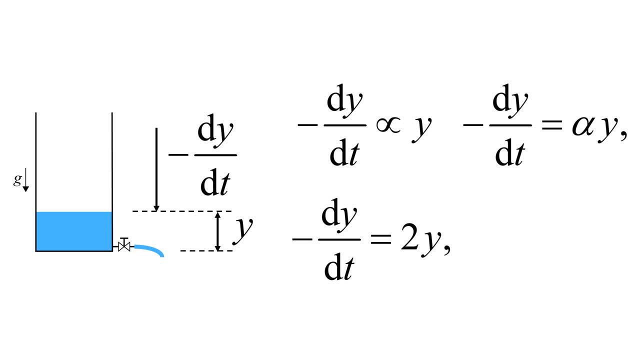 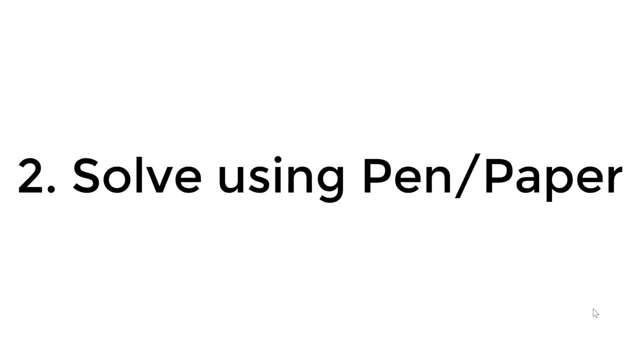 Lastly, since we have the first order ODE, we need one initial condition. In this case, we will need the initial height of the water. I chose 1.. Now let's talk about how to solve. In this section, I will solve given ODE using pen and paper approach. 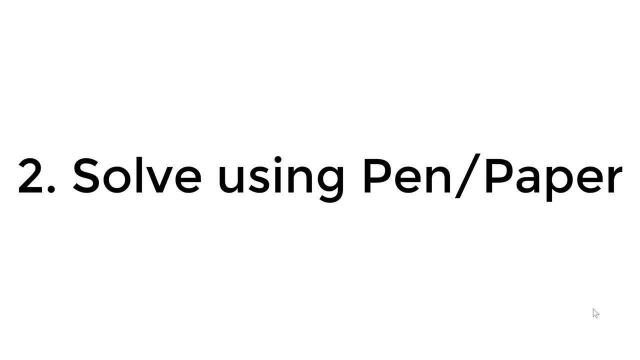 to check your solution from ODE 45 function is reasonable. If you know how to solve it using pen and paper, you can skip this section. Since this ODE is a separable equation, I can move all the terms related to y to the left-hand side. 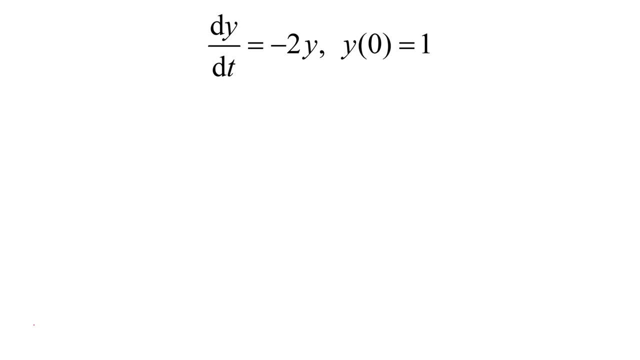 and all the terms related to t to the right-hand side. So I have dy over y on the left-hand side and minus 2dt on the right-hand side. To solve it for y, you can integrate over dy on the left-hand side. 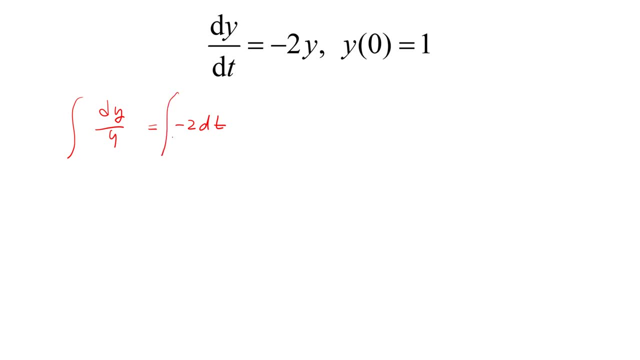 as well as integrate over dt on the right-hand side Using the indefinite integrals, you have a natural log. y on the left-hand side equals minus 2t plus c. c is an arbitrary constant. To express this equation for y, you will have: y equals e to the power of minus t plus c. 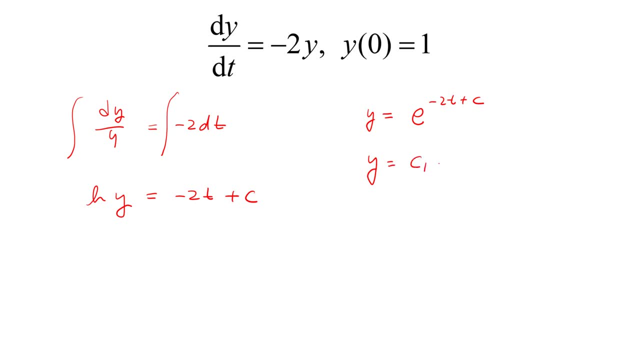 or y equals c1 e to the power of minus 2t. Again, c1 is an arbitrary constant. To determine c1, you can use initial condition y0 equals 0.. To determine c1, you can use initial condition y0 equals 0.. 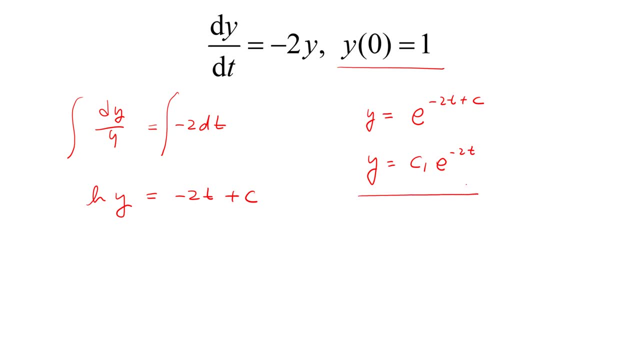 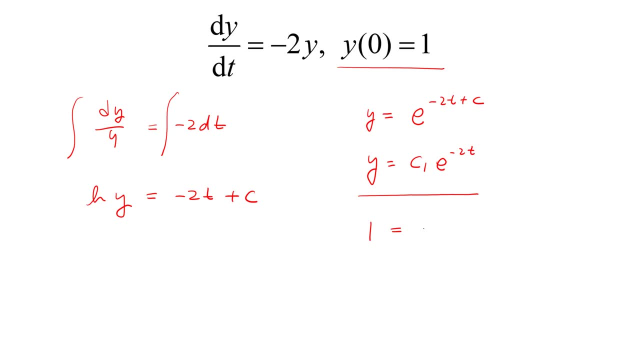 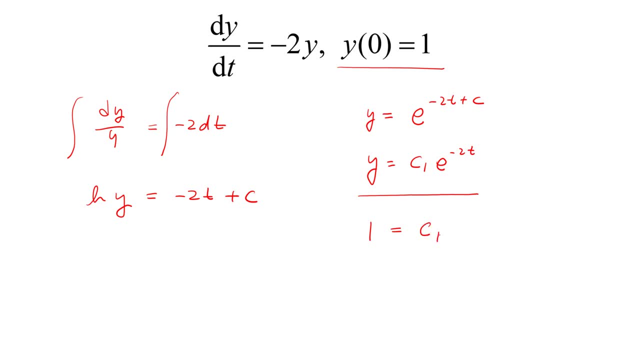 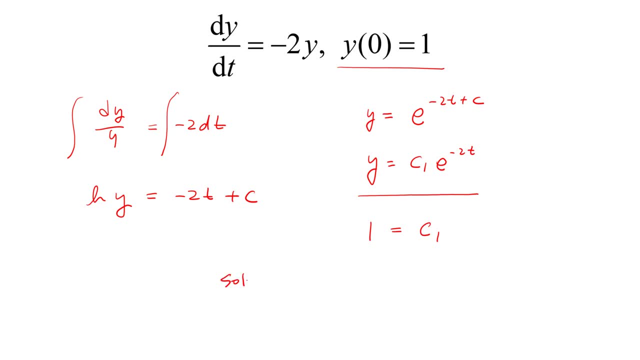 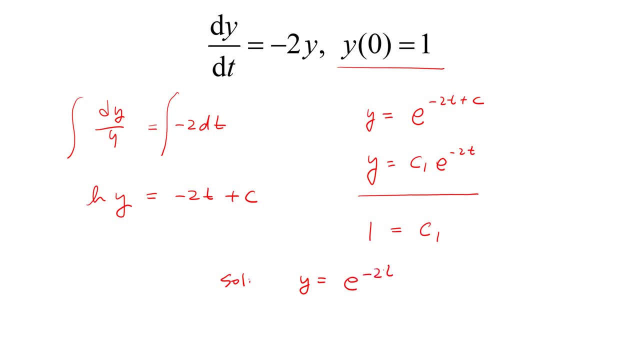 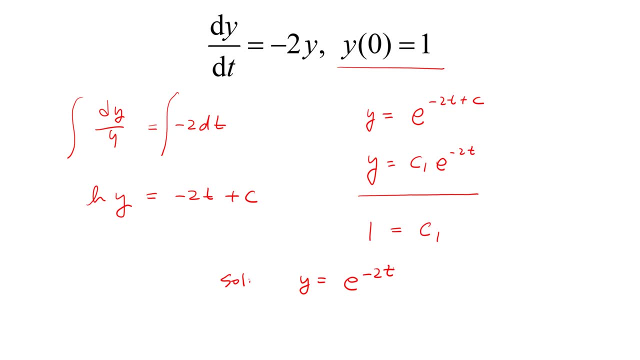 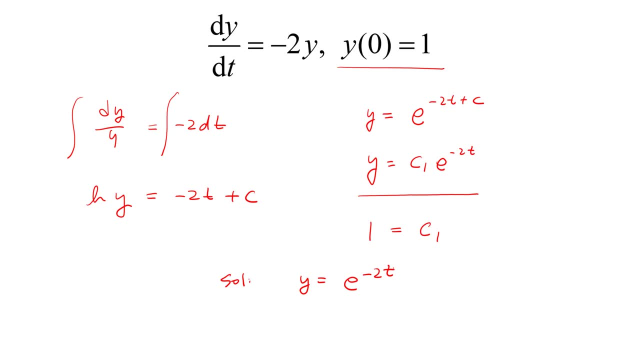 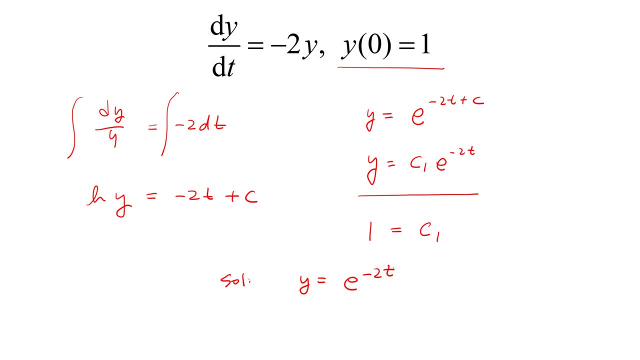 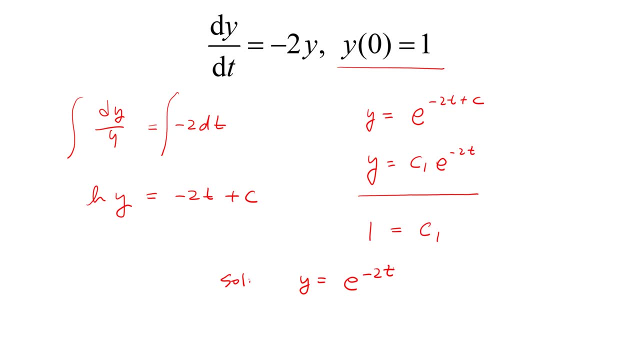 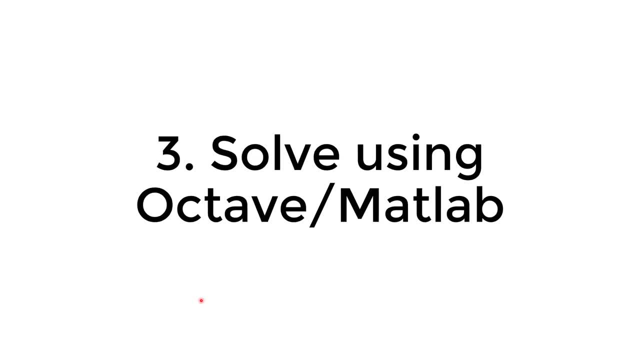 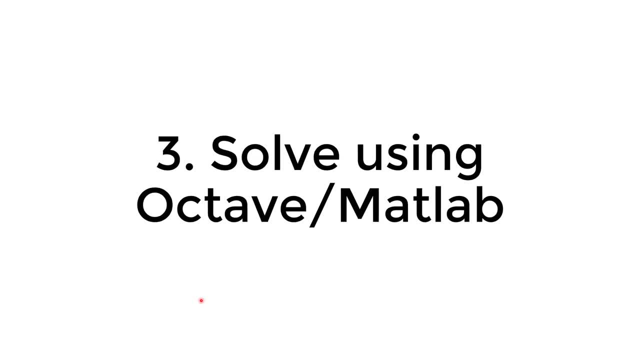 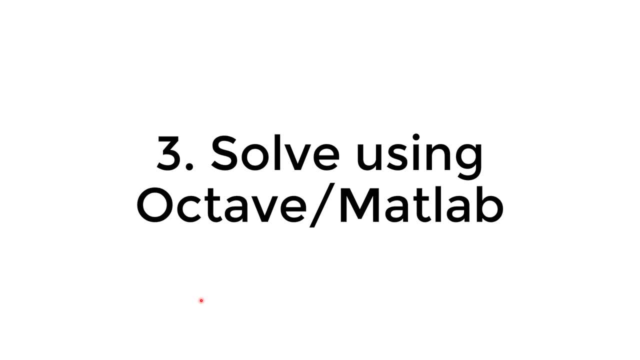 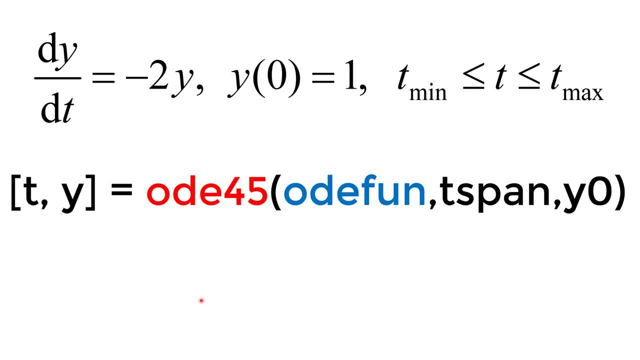 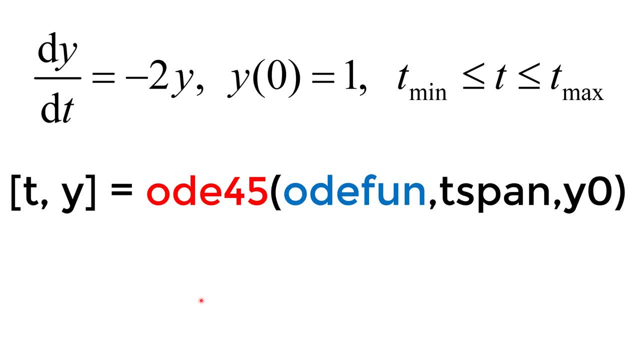 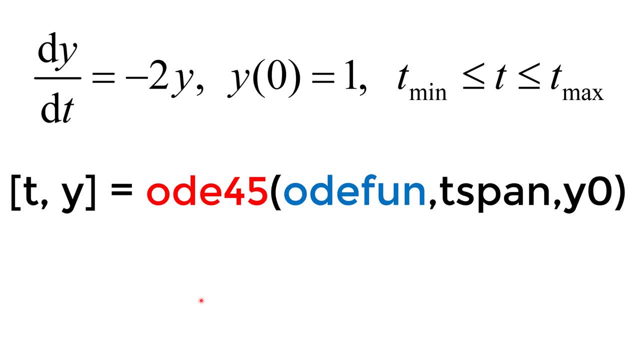 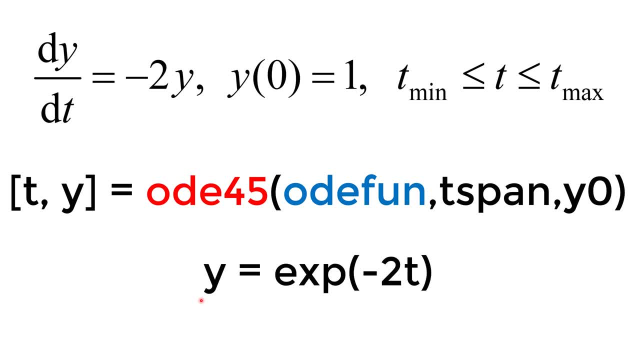 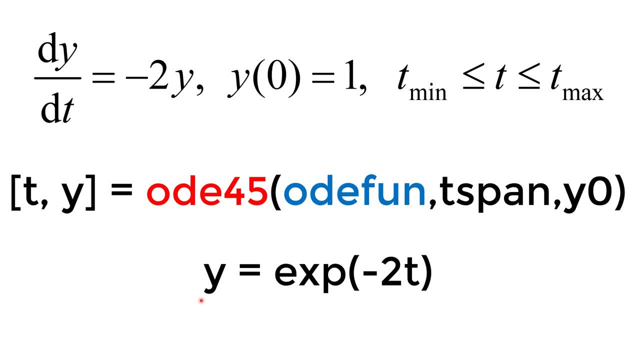 To determine c1, you can use initial condition. y0 equals 0.. The first parameter for the OD45 function requires the ordinary differential equation that you'd like to solve. One way to define is to create a separate m-file. I'll show you how to do shortly. 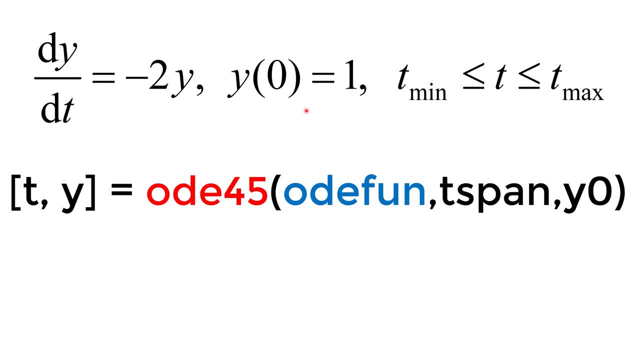 Next, we need to define the range of the independent variable t. I use the t-span as a variable name for a 1 by 2 row vector, And the first element should be the lower bound and the second element should be the upper bound. 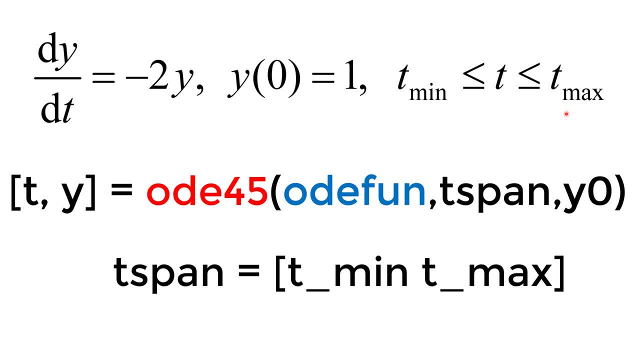 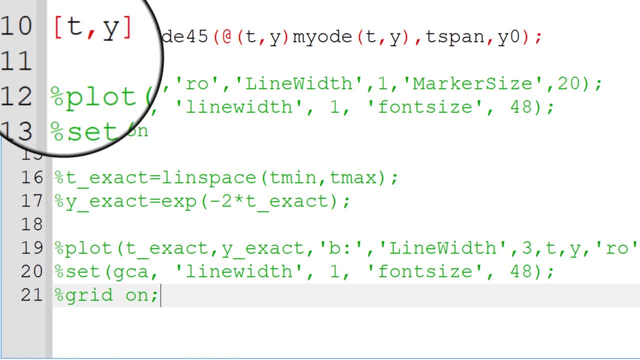 Lastly, you need to define the initial condition y-naught. In this case, y-naught equals 1.. To work with OD45 function, I use t and y as output variables. You can start with ty and square brackets. Next step is to define the variable t. 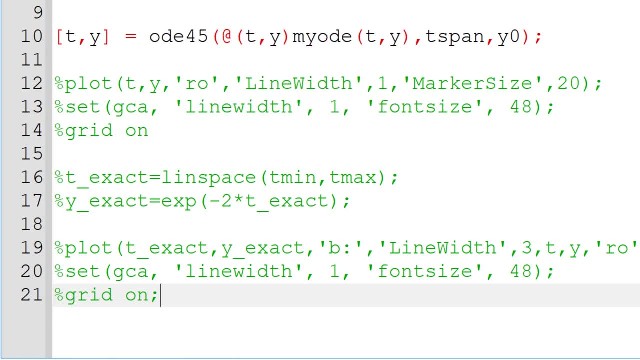 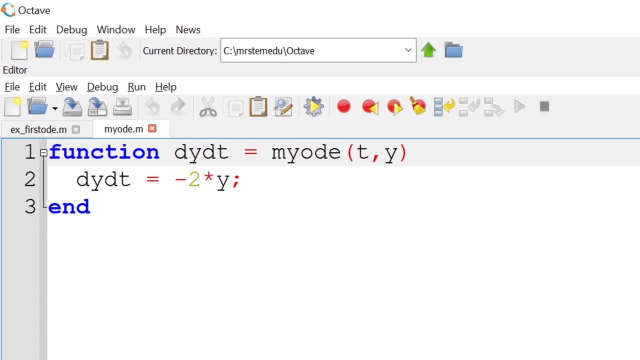 And define the ODE to solve. You can open a blank script And define ODE as a user-defined function. I start with function, followed by the dy, dt as an output And function name myODE and t and y as arguments. 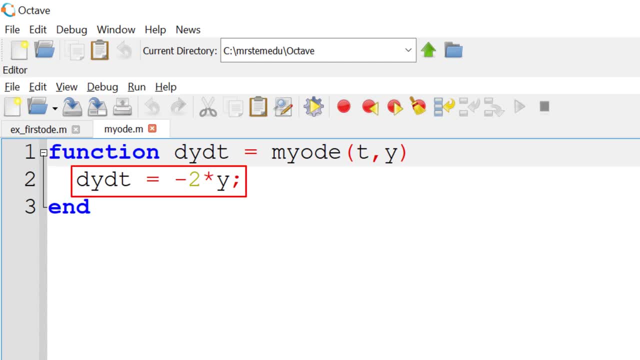 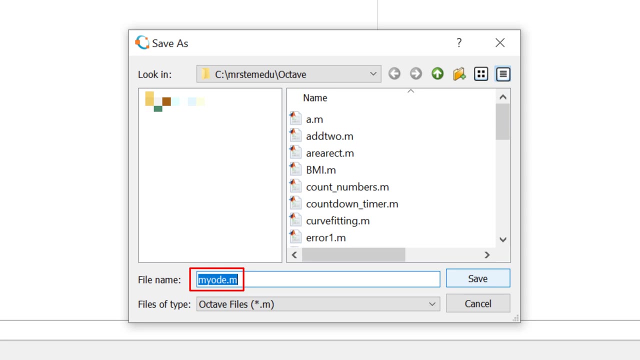 myODE is dy over dt equals minus 2y, So I typed accordingly. Then I wrap up with end at the end. Save this script as the same function name, myODEm under the same working directory. So myODE45 function will call myODE without having a problem. 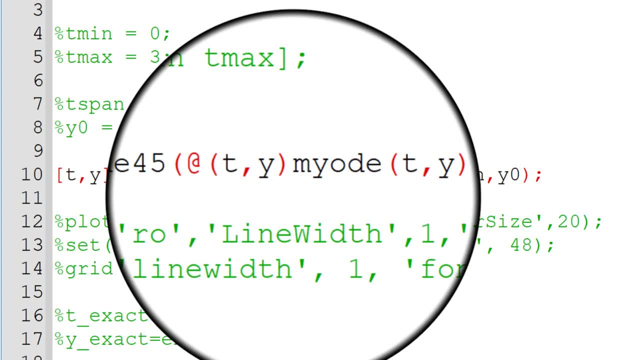 To call myODE from OD45 function, I need to start with at, with parentheses, Basically telling that myODE is a function of y versus t, followed by the function myODE, with parentheses. Then I need to define the range of the time, t, to work with. 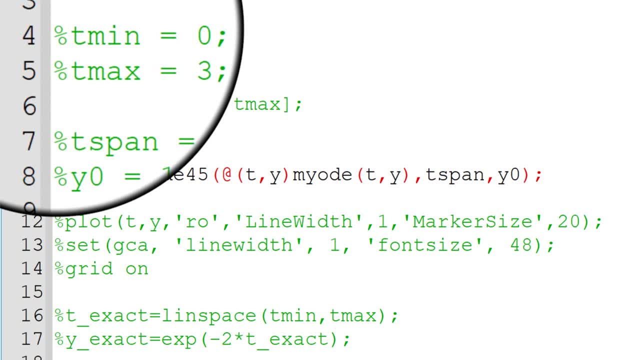 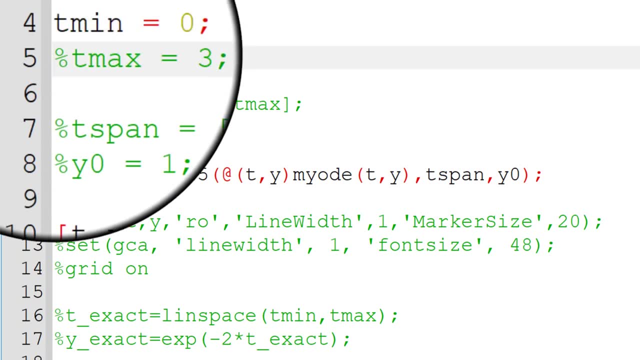 I chose 0 for the lower bound and 3 for the upper bound, So I use: tmin equals to 0 and tmax equals 3.. To fit them into a single variable, tspan, I use tmin and tmax with the square bracket. 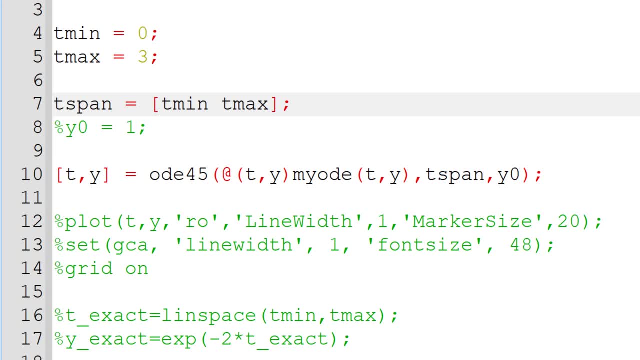 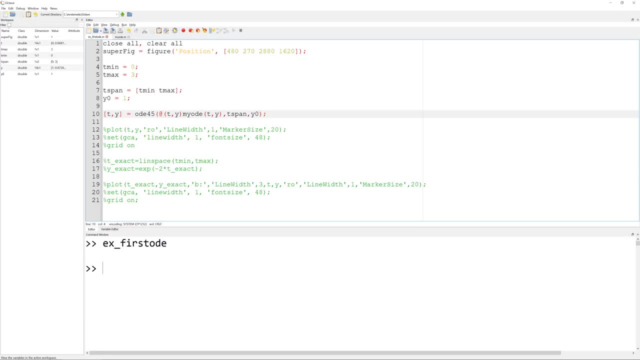 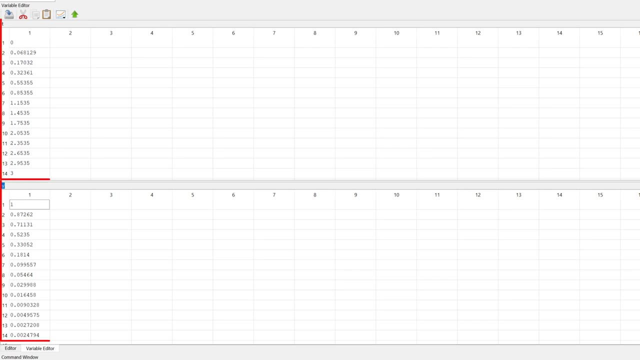 Lastly, you need to define the initial condition y0.. In this case, y0 equals 1.. When you solve the ODE, ODE45 will return the solution as a row vectors for y versus t. As you can see, you find two row vectors in the variable editors. 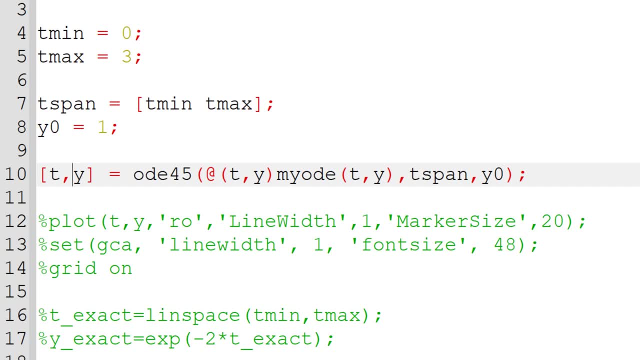 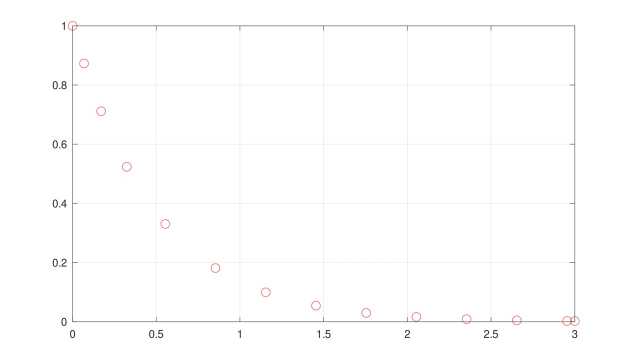 To visualize the data you can plot using plot function, I use the wrapped empty circle and increase the font size and add the grid. To double check if this solution is reasonable, I would compare with the analytical solution: y equals e to the power of minus 2t. 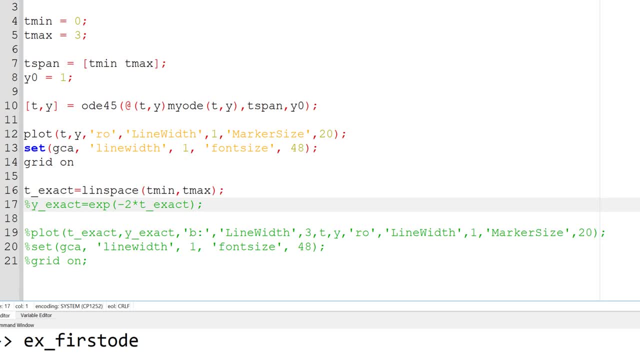 You can create a separate row vector for the time, at the same time range from 0 to 3, t exact And then create the y equals e to the power of minus 2t. for the plot, You can add the analytical solution to the existing plot for the comparison. 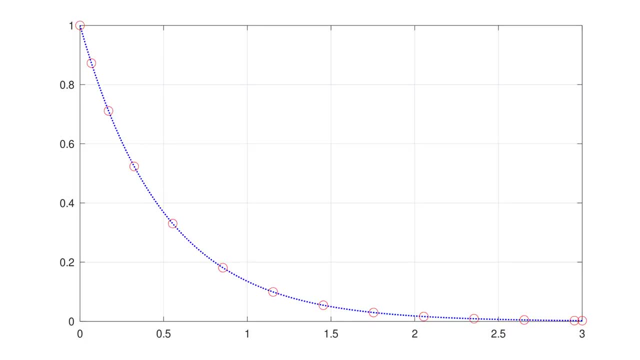 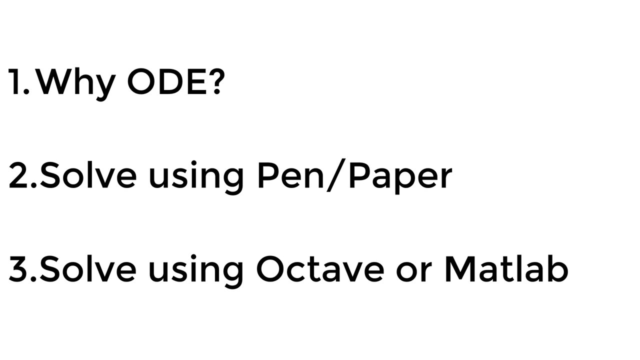 As you can see, two solutions agree to each other, which means that ODE45 solved the equation reasonably. In summary, we briefly talked about how to come up with ODE, Followed by pen and paper approach, and ODE45 function in Octave and MATLAB.